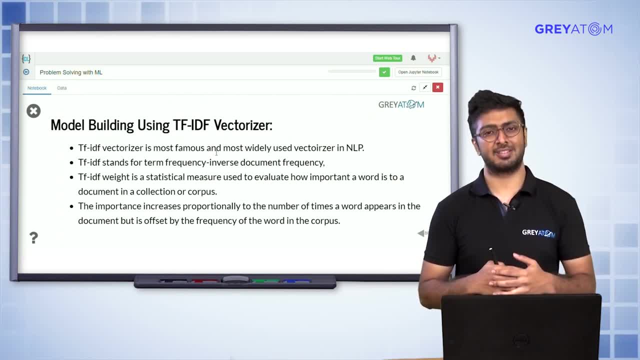 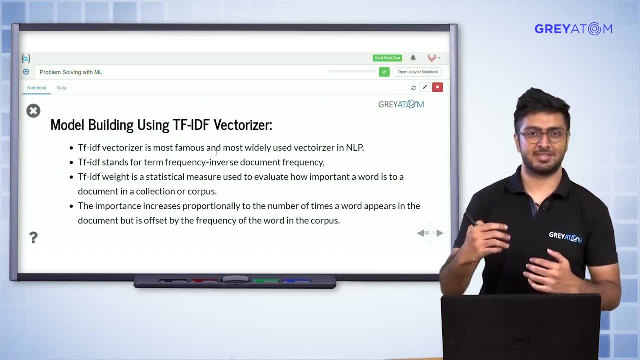 the doesn't say anything about that, whether it belongs to an author class, whether it's about the task about predicting sentiment, just because the word the occurs probably 10 times, 12 times, 20 times in each of the document, it probably doesn't say anything. So the idea is that 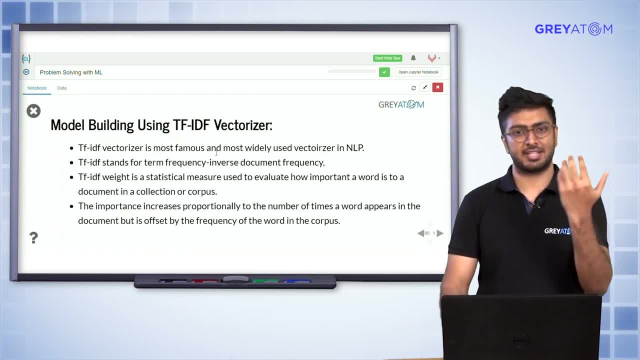 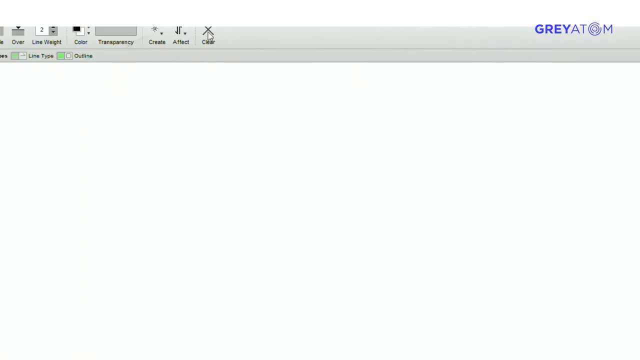 right now we were using counts right each time. what is the count that? so right now, if we have our data, So I will just kind of explain this. So right now, you basically had something like this, where you had this feature: X1, which was basically the presence of the word the and it's count, and X2 was some other. 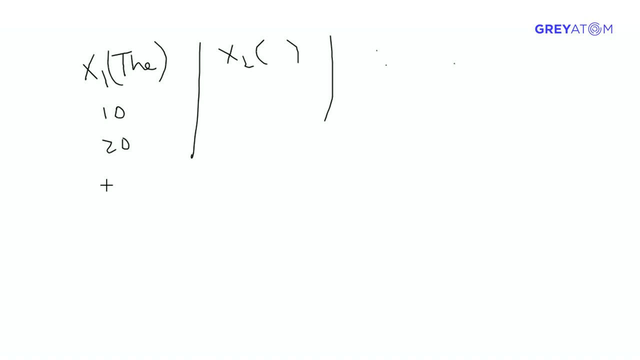 word and so on and so forth, and this is 10, this is 20, this is 30, and so on. Now, this probably occurs in each word: 10, 20, 30 times each document, basically, and we can clearly see that the presence of this, just because you can clearly infer that this word is getting repeated in each of the 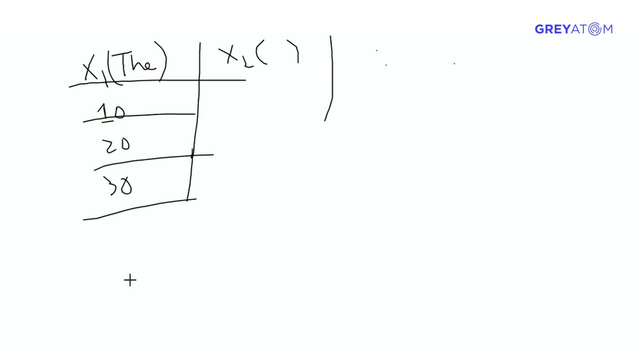 document. probably that means that this word has no significant contribution to the sentiment right, because it was say: you're doing sentiment analysis or you're probably doing the same author classification. So probably the word the has been used by an author 10 times doesn't say anything about. 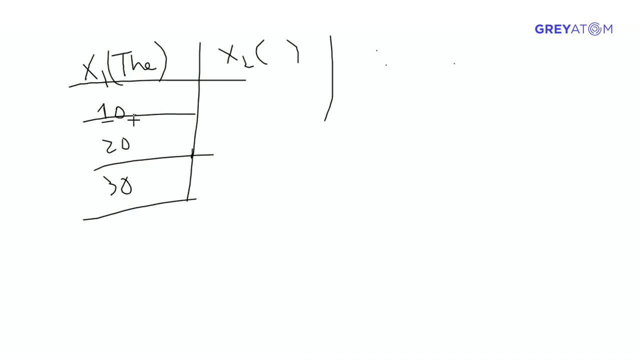 that author as much, because it's kind of getting repeated almost. you know it's getting repeated every time in each document. but say probably the word finance right, So probably finance has been used by this author. say two times this author has used zero times this author. 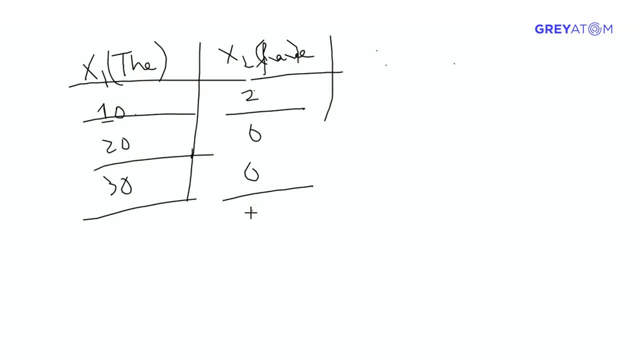 has used zero times, and then some other other author, So there are probably used five times right. so that probably says that this authors are someone who probably write related to finance. So that's the idea that what we kind of want to capture is that currently, in this way, when we are doing count Vectorism, when 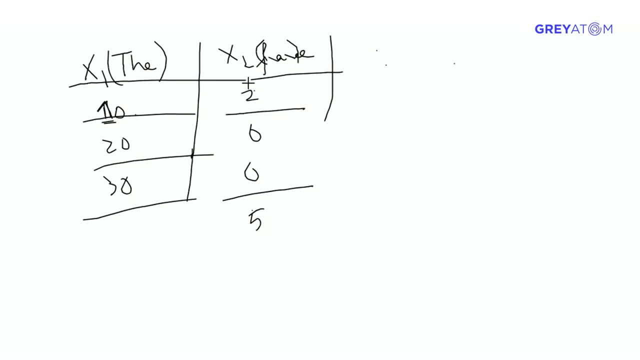 we are counting if number of times the word the has occurred in a document, we are not really giving equal weightage of both the word the as well as the word finance. right, we don't want to do it. what we got to do is not give it a weightage. this weightage We 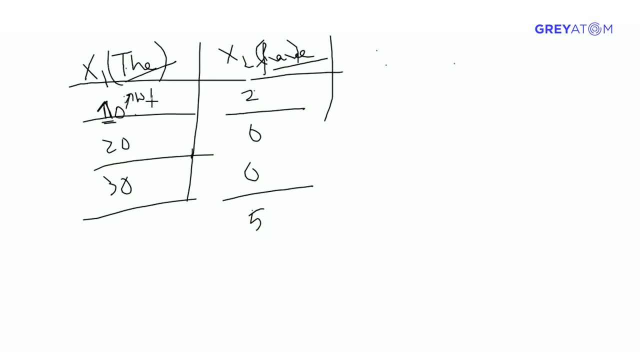 want to give it a weightage which is low, so w, which is low, and we want to give it a weightage. okay, this is what we're going to give- a weightage which is high, right, so that's what we want to do out here and that's the concept of tfid. and what is a weight? the weight is something which is 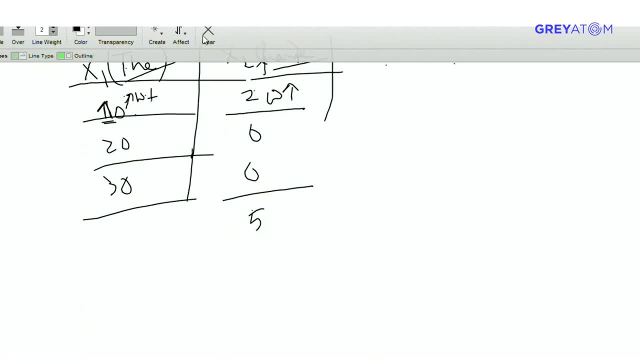 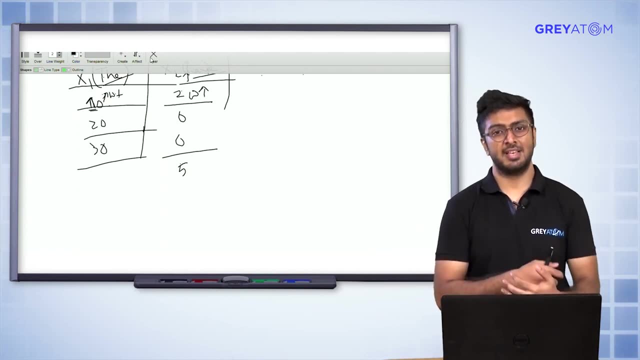 basically based on the fact how many times that document occurred in other documents. if the document- sorry, how many times the word- occurred in other document, if some word is basically occurring in each document, it's since there are thousand documents and each of the thousand document it is occurring in each of those documents- then probably give it a very low. 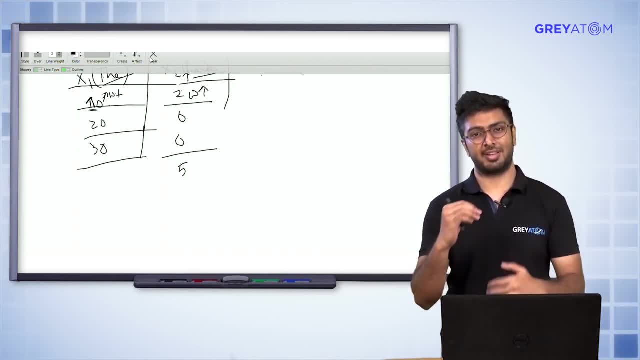 weight: probably zero, right, and if there's a word which is probably occurring in, say, five documents, then probably give it a higher weight. that's the idea that we are going to use to, kind of, instead of using just directly counts as it is, we are going to give that some weighting scheme. 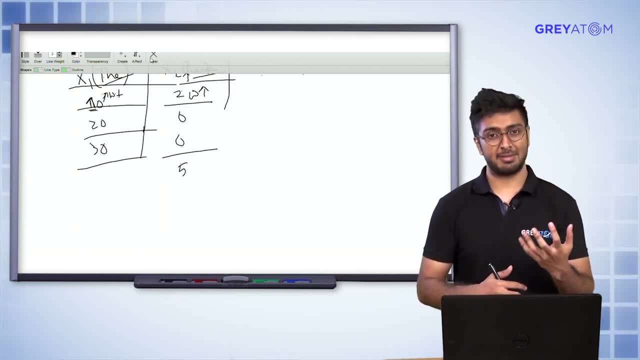 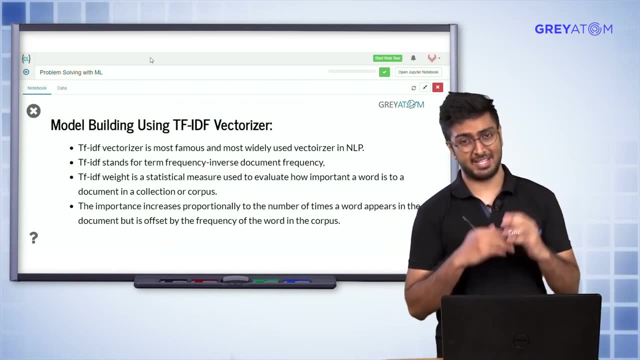 right. so we are going to give weights to each of those counts and the weights are basically being decided by how many times that particular thing occurred in other documents. you? so that's the concept of tfidf. so basically now breaking it down, tfidf basically consists of two. 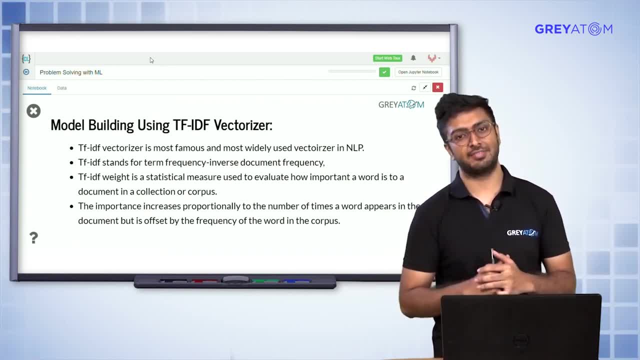 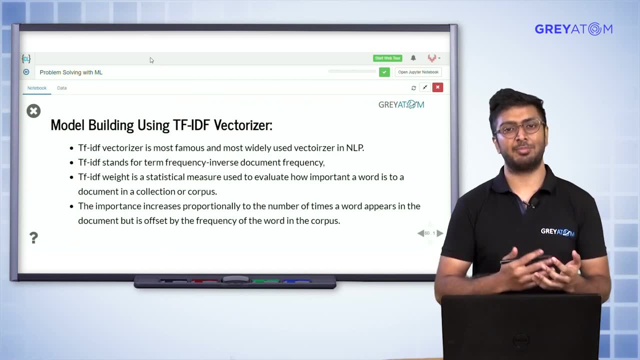 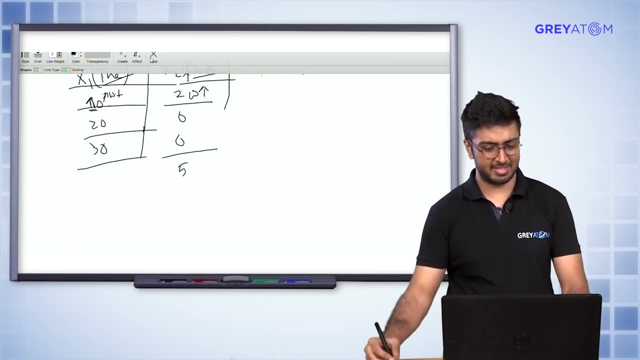 parts. term frequency, which is tf and idf, is inverse document frequency. pretty clear to you guys. term frequency is something that we are already familiar, which is basically count by total number of words in that total number of words in that particular document. so count is basically so count. is this 10? now if, say, this particular document has say 30 words, right? 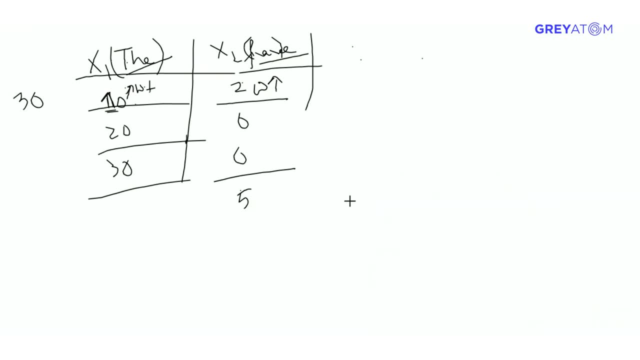 so if the particular document has 30 words, so the frequency is 10 by 30, which is 0.33. so this has 2 by 30, right? so that is your frequency, so count. and this say: had 40 words. so out of 40 that was 20 was the and out of that 0 by 40. so that's the idea of frequency, so frequency is count. 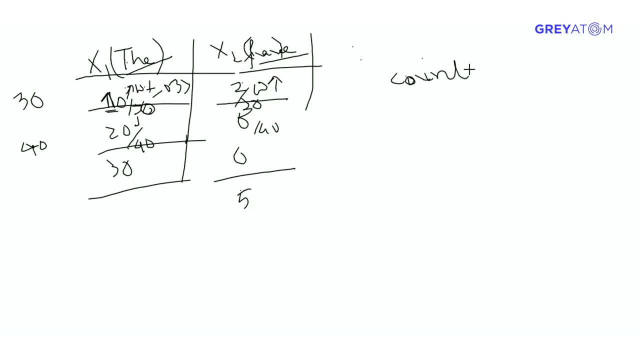 is, is, is count, is is tfidf by number of words in doc in that document. this is my frequency right, so this is called term frequency. term frequency is nothing but count by number of words in that document. now that is it. and inverse document frequency is something that we need to understand, which is basically. 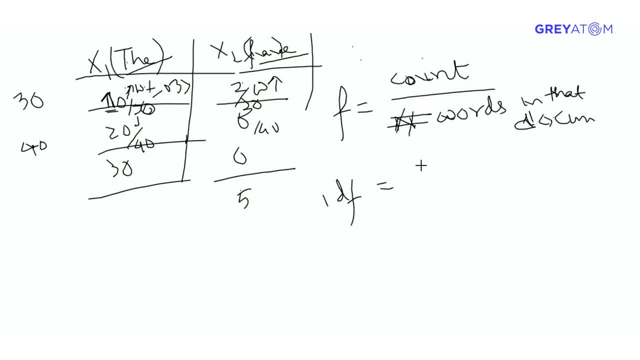 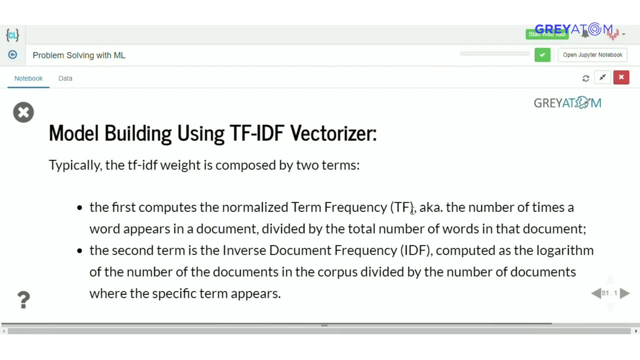 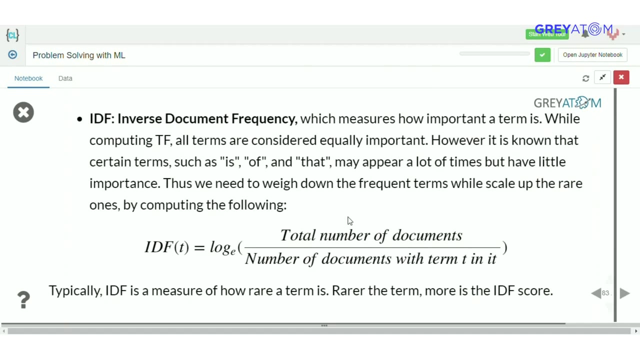 something which kind of penalizes weights for the number of times it occurs in other documents. so now, so I have already explained you, so. so what is all you need to understand is this term. frequency, I've already told you. inverse document. frequency is this particular thing: log of total number of documents. 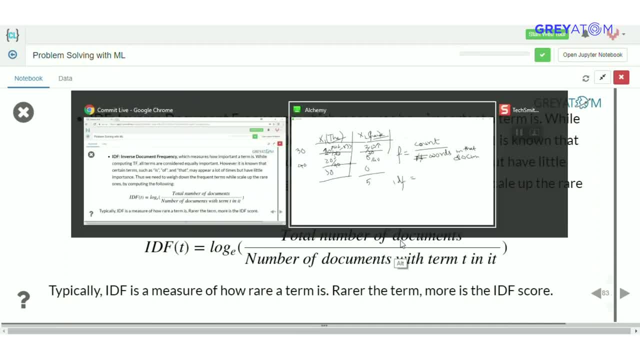 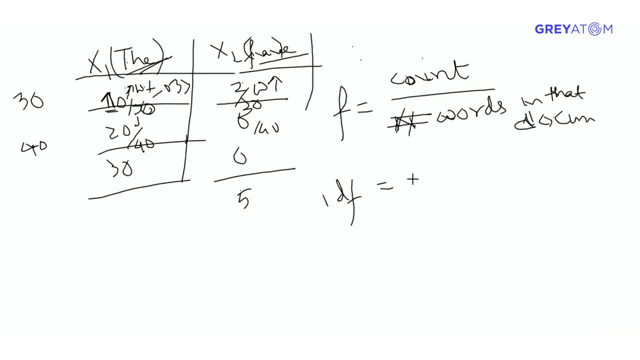 by number of documents with the term T in it right. so basically for each term, each, this particular word, the, you would have an inverse document frequency, which is basically log of number of documents by number of documents which has word though at least one, one word though at least has got word the one in once in that document. 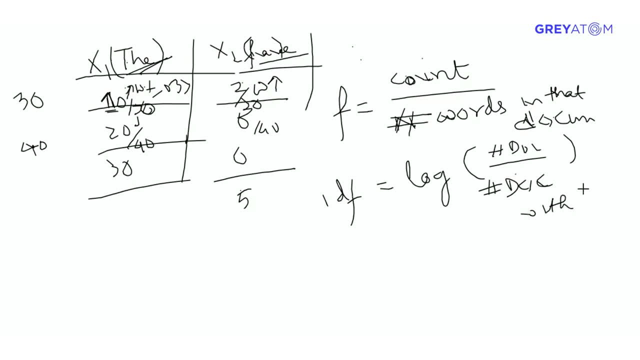 right, so that's it. so obviously you can see if there's a particular word which is occurring all the time, so that's it. so obviously you can see, if there's a particular word which is occurring, all the documents. so it basically would have inverse document frequency, number of. 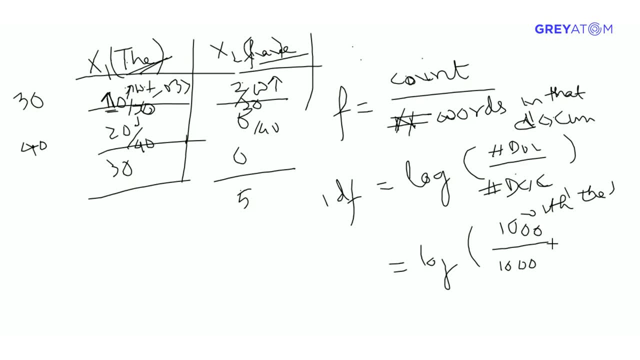 dogs is a thousand by thousand rights. so log of one is zero right. see this particular word which has awkward say only once. now let's consider one word which has probably offered just once in one document. right says is log of thousand, which is total number of documents by one, so that is log of. 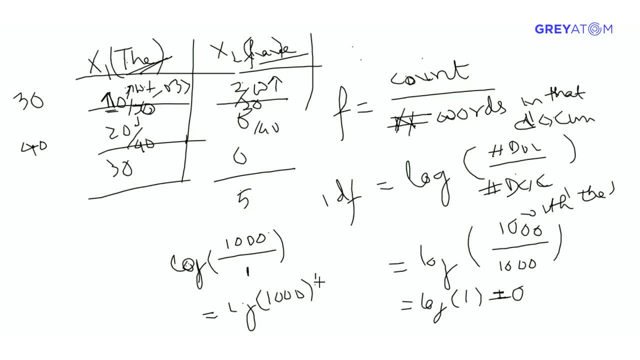 thousand, which is probably a very high number. i don't know probably if it's log base e right. so this is roughly eight point something, nine, nine point something. so that's a high rate. is that you kind of give to something which is uh, which is a word which has just occurred in once? 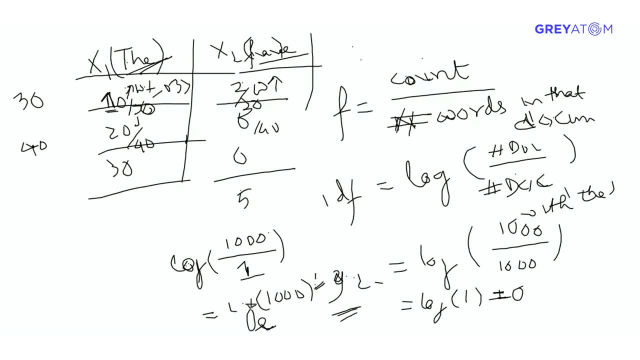 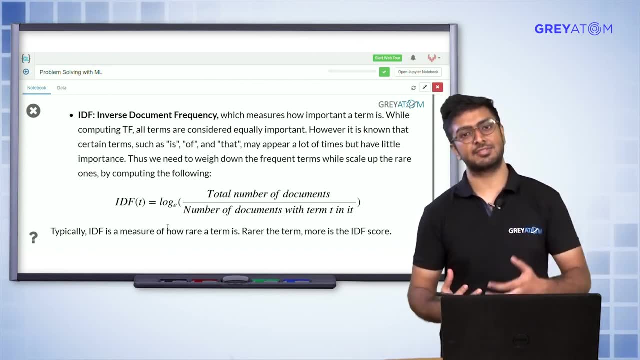 in one document, right, so that's the concept of term frequency and tf idf, right, so tf idf is something uh, which is uh, basically giving a weightage to words that are occurring a lot less in in across documents and giving a lot of low weightage to document to words which are kind of 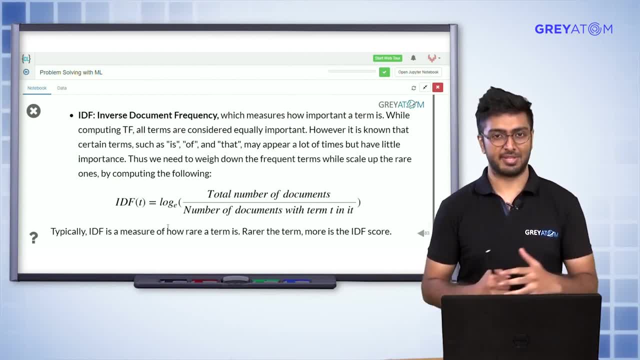 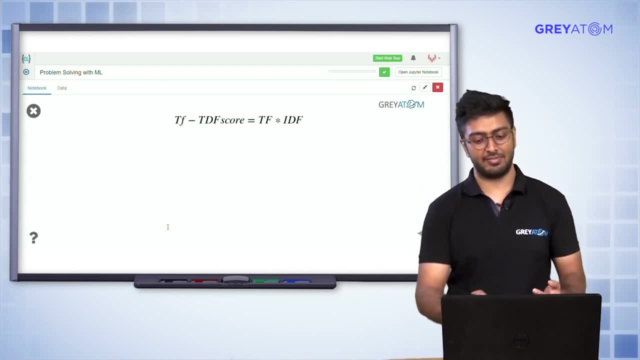 occurring a lot more in across documents. right, so that's that's the concept behind tf, idf. so how do you kind of calculate tf? idf score is basically tf into idf, so tf is something that we are already familiar with, which is basically what count vectorization was. 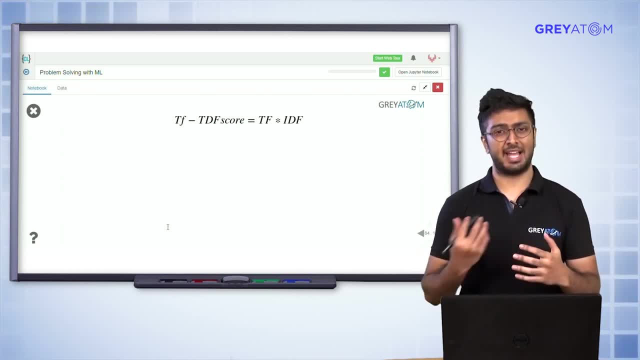 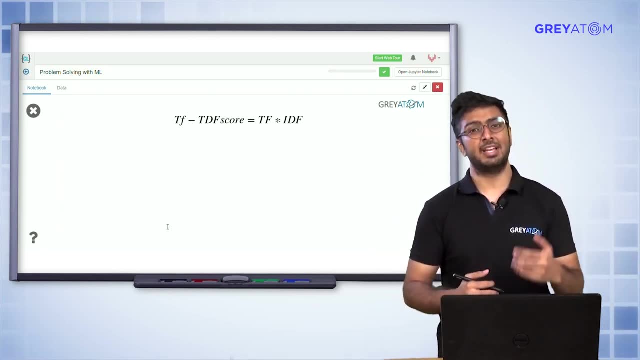 doing almost, and to that you basically add a weight which is not add. you multiply your weight to that which is basically the idf. idf is log of number of documents by number of documents that particular word has occurred in. so obviously this weight would be high for weight documents which? 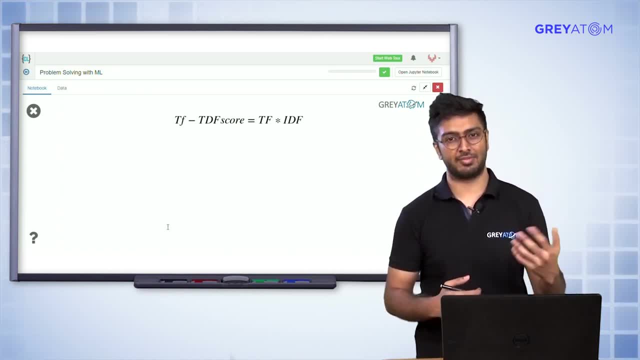 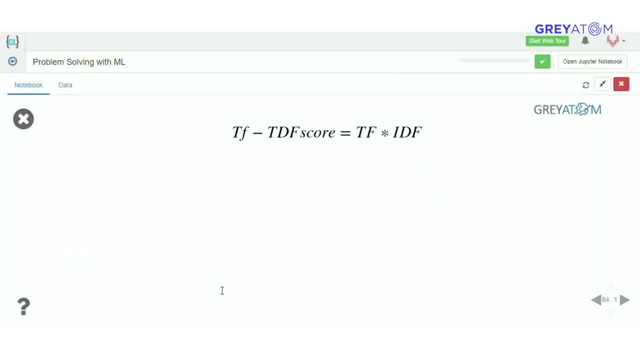 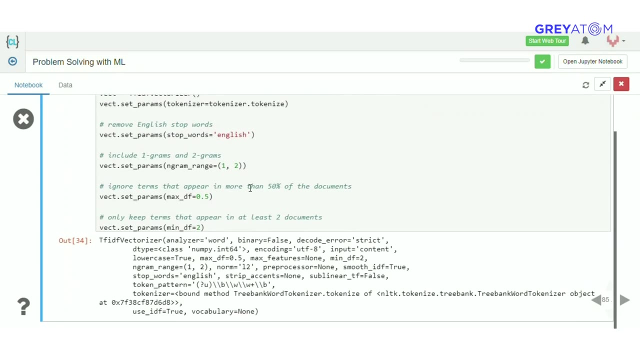 are basically word, words which are basically occurring just in couple of documents, a very less number of documents, and this weight would be extremely low for words which are basically occurring across most of the documents, because that probably doesn't have a lot of significance and that's it. so now you kind of do the same thing that you did earlier. so instead of importing, 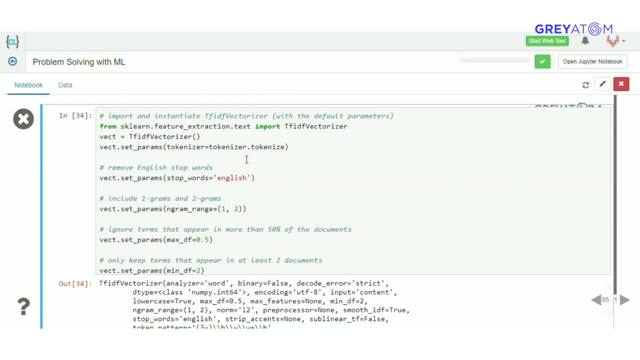 count, vectorizer, and doing all of the things that you did. you basically do the same thing now, you again. you just import tf, idf, vectorizr, you initiate the class and then you set the params right: what it's the staming you want. what is the lemmatization you want. what is the stop word removal you want. 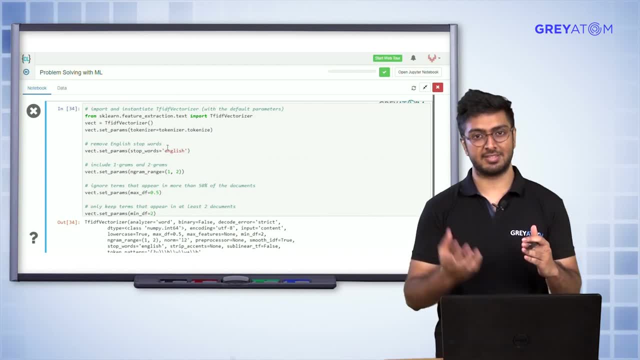 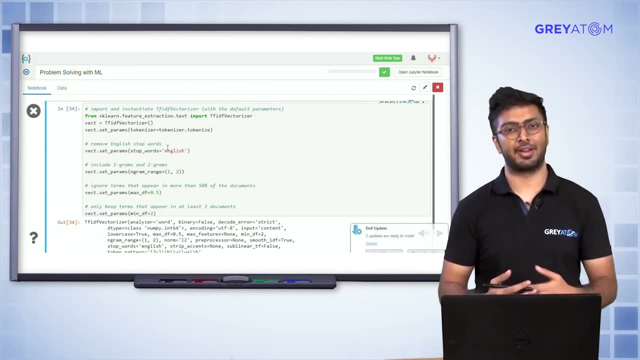 and the number of words that need to be there for it to be even considered as a feature. and if, what are the number of words that? probably, if there's a word which occurs in hundred percent of the documents, probably you kind of remove them, right. so those are the things that you kind of still do. 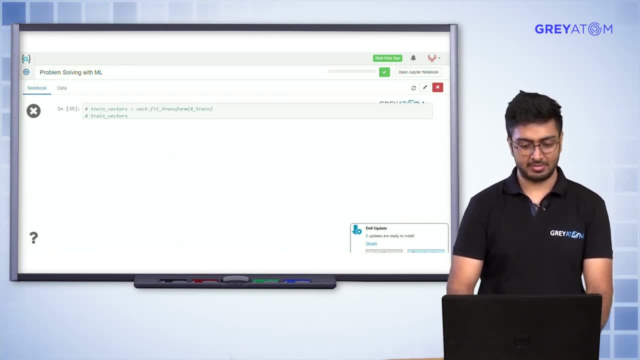 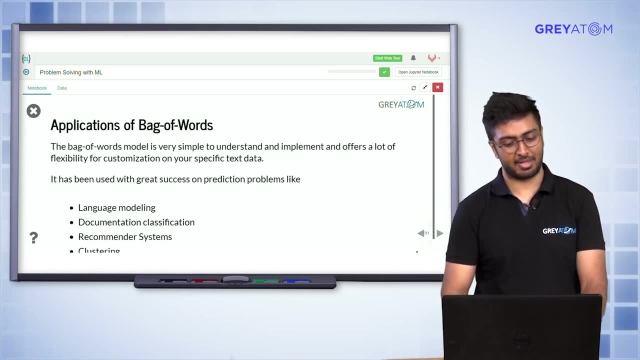 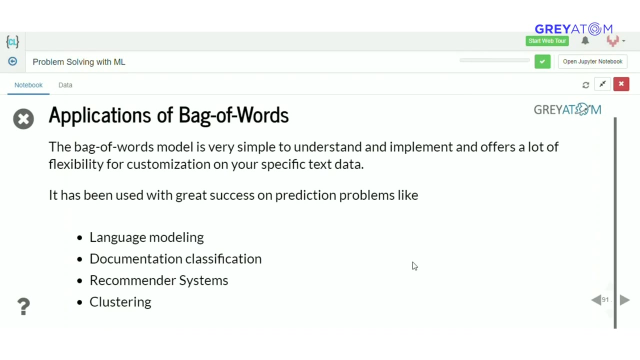 and once you do that, then the rest of the thing is pretty simple, right? so just you go out, build your model and then you just do the same accuracy prediction. so that's about its applications of back-of-watch model is, I think. I think it's fairly. yeah, it's. it's definitely not an overstatement to say that it's. 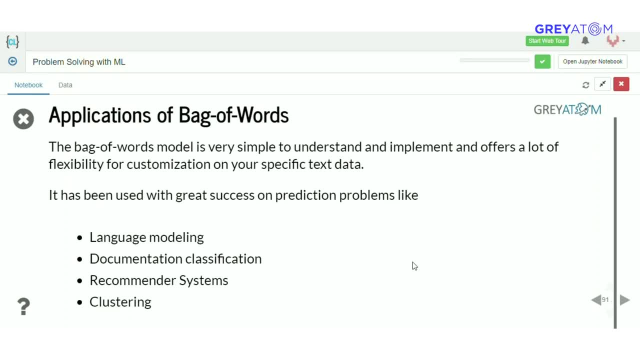 probably there in across 90, 99 percent of the text classification tasks. that are, yeah, basically a basic level text classification tasks across industry. you would definitely go any places Kaggle. you see a lot of them use back-of-watch obviously, that kind of obviously. by now you kind of get that, that just doing. 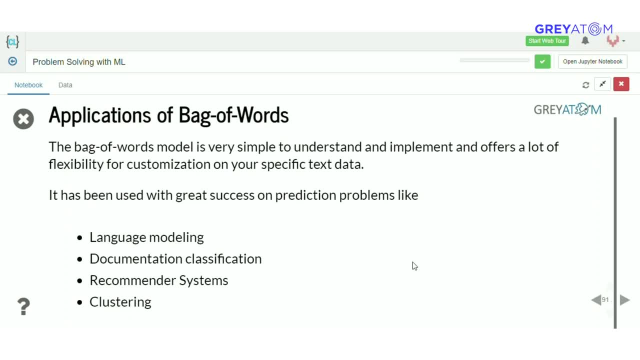 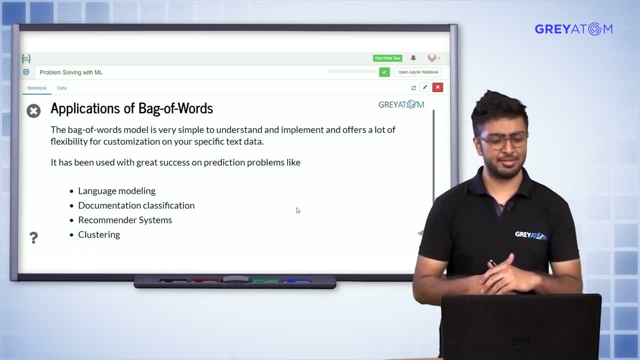 back-of-watch would not get you really a lot of places. you have to kind of be very smart about it in the kind of features that you want to do and all of that. so in whatever things you do right in in back-of-watch, you have to be very smart about it in the kind of features that you want to do and all of that. so in whatever things you do right in in back-of-watch, 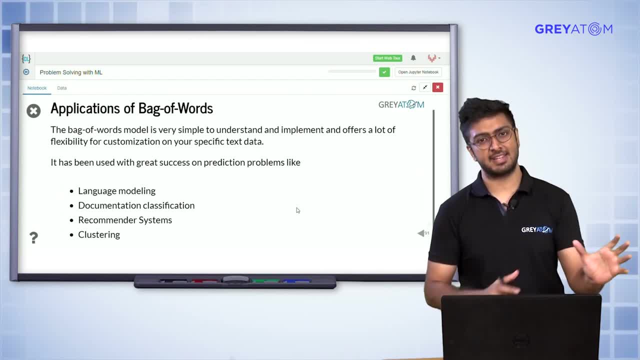 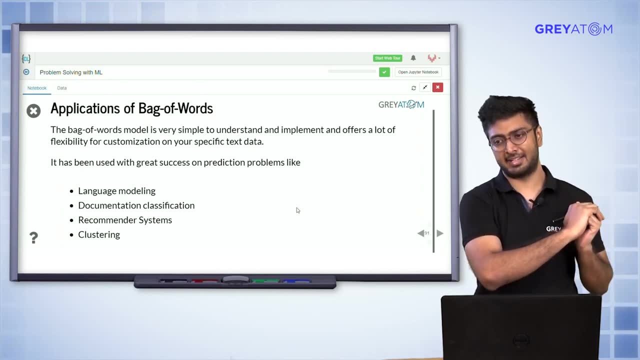 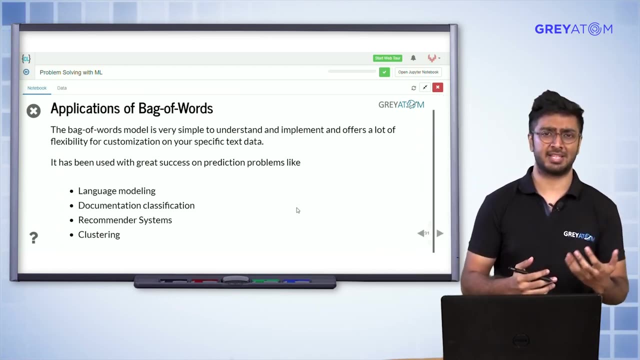 back-of-watch is basically this concept where you take a text and convert that into a numeric representation, and that is something that is applicable across and, as I said, I was 99 percent of X domain NLP related tasks that you would do it, whether it be supervised learning, whether it be something else supervised. 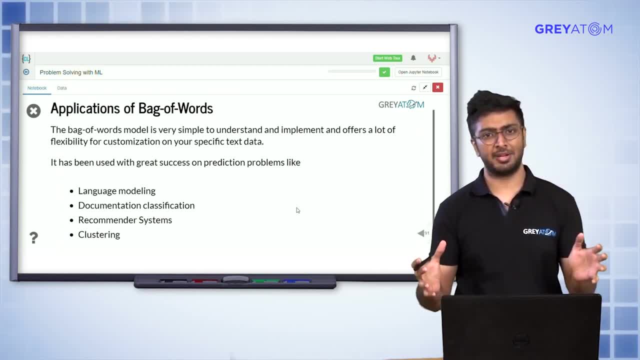 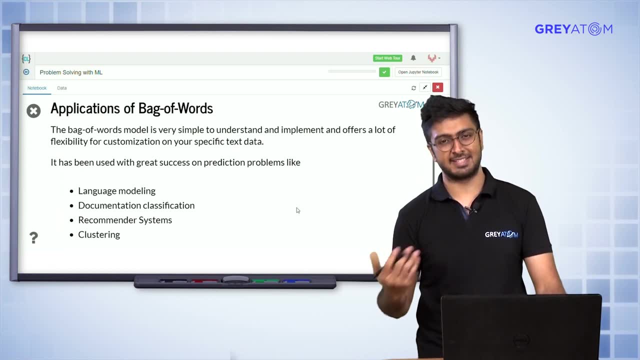 learning is basically just the part where you're gonna take, convert that into a numeric representation and then you just do the whole. you know the whole training and testing thing that you're going to do and then you just do the whole. you know the whole training and testing thing. 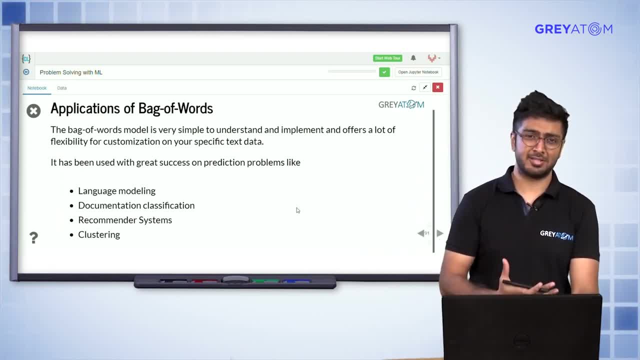 that you normally do in other parts. but in any case you want to do unsupervised things like information retrieval or clustering or recommender system. you have still got to use TF, IDF and to represent. take your text and represent that in a numeric form and then do the same things like in clustering you to 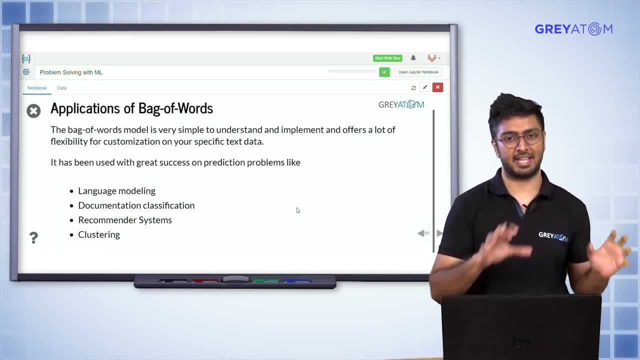 kind of cluster that into different buckets. if you want to cluster text into different buckets, you first have to convert text into a numeric representation using this- what I've explained- and then you do the rest of the things, which is something you're familiar with. so obviously there are a couple of 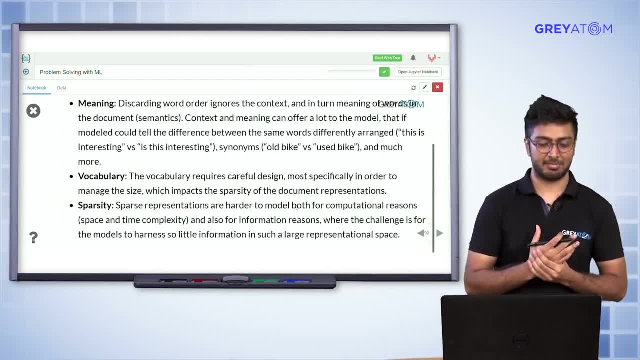 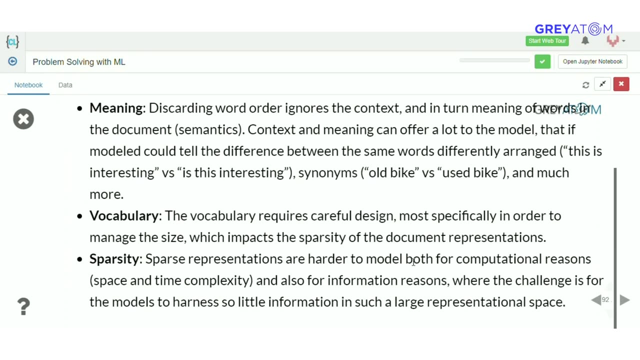 limitations with bag of words. firstly, is this whole concept of meaning right, semantics and context that is not completely captured right. as I said, not good is one example I gave you about negation. so negation is one example, but there are a lot of other ways where the context of the words right. so basically, 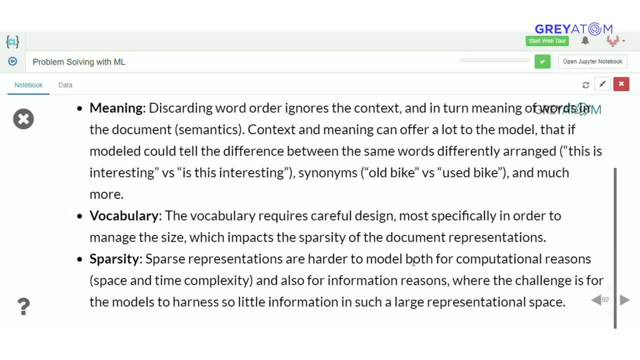 when I'm saying this is good, right? so what this particular word this refers to, right? so all of those kind of things are basically a problem, right? so? old bike versus used bike, this is interesting versus, is this interesting, right? so those are very different context that you kind of see. so those kind of examples are something. 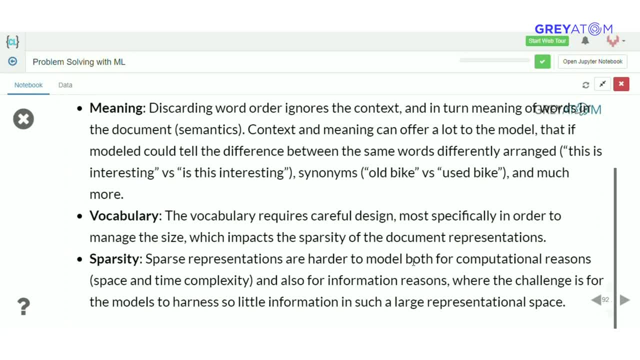 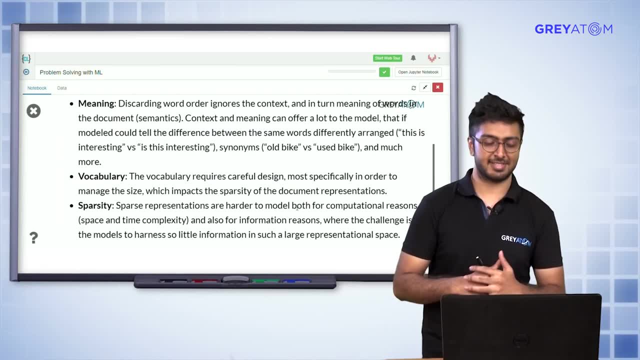 that you cannot kind of capture using because in both the cases, say this particular example, let's take this example, this is interesting or is this interesting? so this is interesting is a fact. is this interesting? is a question. there are different context that you understand. now, if you look at the bag of 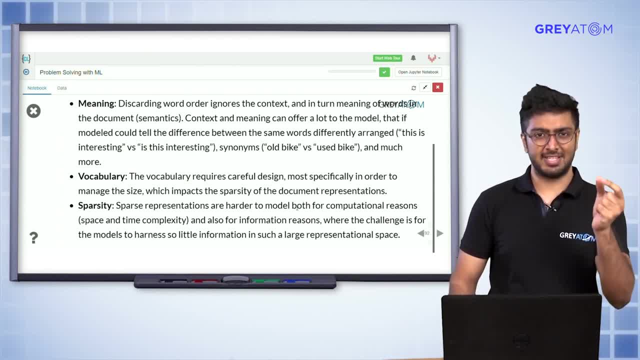 words, representation for both of them. it would be exactly same right. if is is what occurring in the world, it's probably count of it is one. this is a counting, count is one. interesting is occurring count is one and it is the same for both the cases that we have discussed here. the thing to kind of 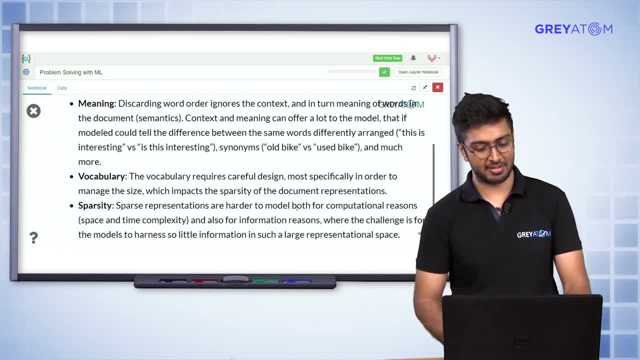 understand, that is, but the context are different, right? so those kind of things, those kind of cases, are something that you kind of completely, completely miss out using a representation like bag of words. that's why you need something which is slightly more smarter to do that. secondly, the vocabulary. right. so, as 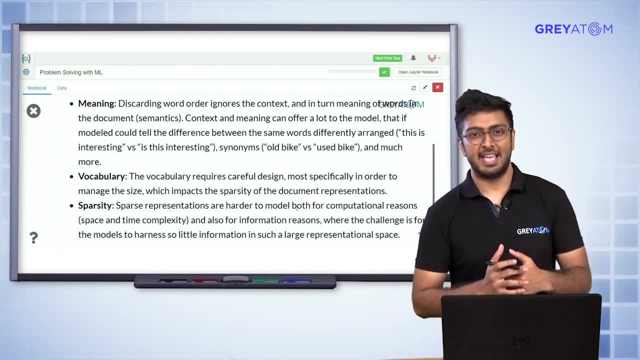 I already told you vocabulary. if you're just using bag of words as it is, it's probably not gonna go a lot of places. you have to kind of smartly design it and what is the kind of vocabulary that you want to use? whether you want to have 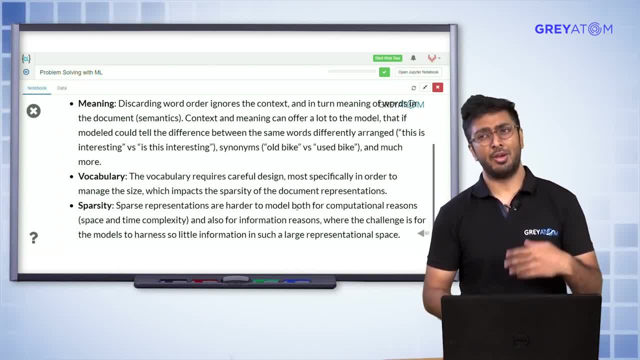 dollar related numeric representations in your features or not? what kind of features you want? you not at all. what numeric features do you kind of want? some certain kind of numeric features with certain kind of other text features. that's the other problem that you have. another third problem which you 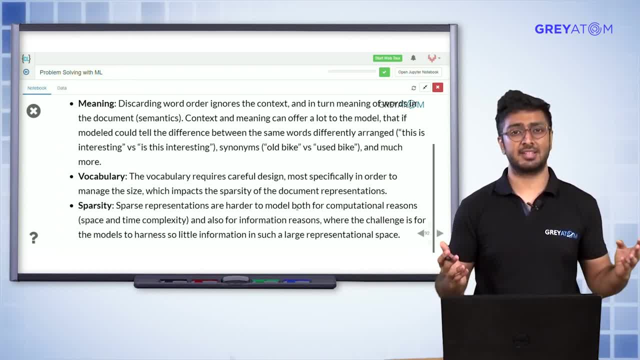 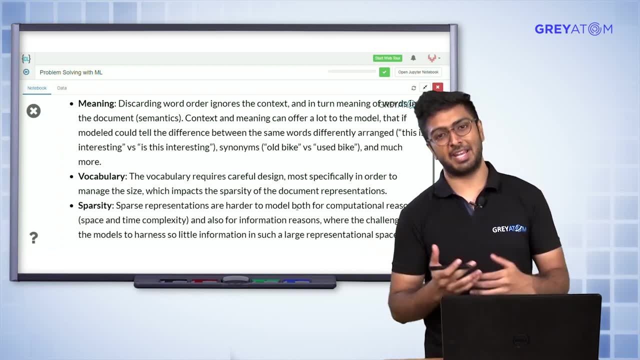 have is sparsity, which is something that we have already talked a lot, which is basically the point that if you're using bigrams- right, and definitely let's not talk about trigrams- so if you're using any of this sort, right. so number of features that you've come up with is extremely huge and it's 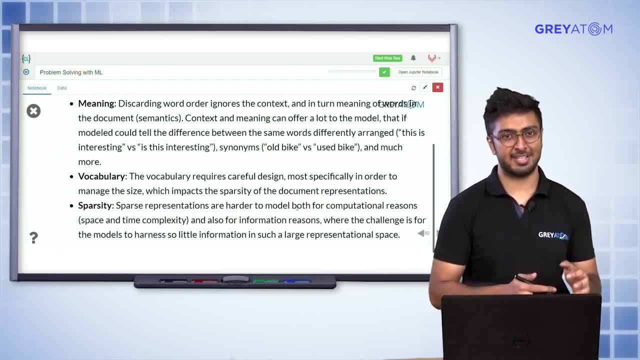 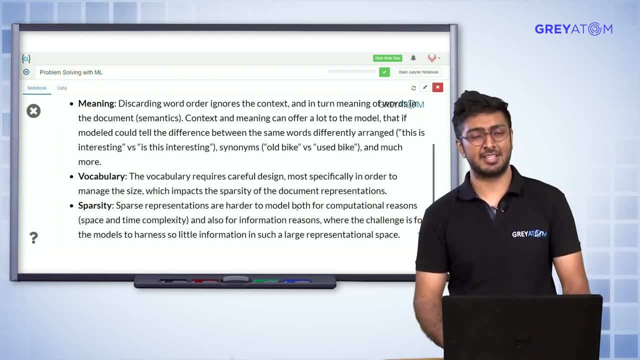 computationally not the most efficient thing, right? so in this particular case we still have 2500 or so, not 25. we had 500 odd examples, right. but saying this, but in cases where you want to kind of classify, it's a thousand pieces of text. 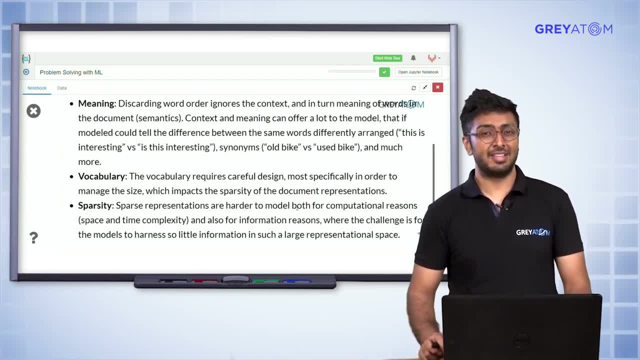 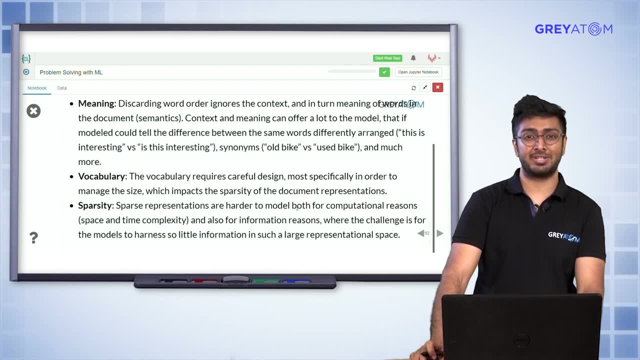 or ten thousand, I don't know fifty thousand pieces of text in those kind of cases. just imagine the number of features that you would kind of come up with, right, with just five hundred examples. you came up with twenty seven, four, ninety two, some features right. imagine the amount of X features that it. 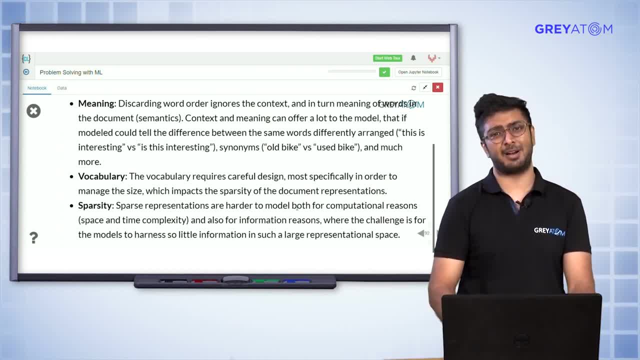 would come up and that would kind of lead to extremely, extremely sparse matrices and dealing with sparse matrices, stuff that we already understand right, because all this distance calculation, all of this kind of gets gets a shot. so definitely sparsity is something that kind of is a problematic. 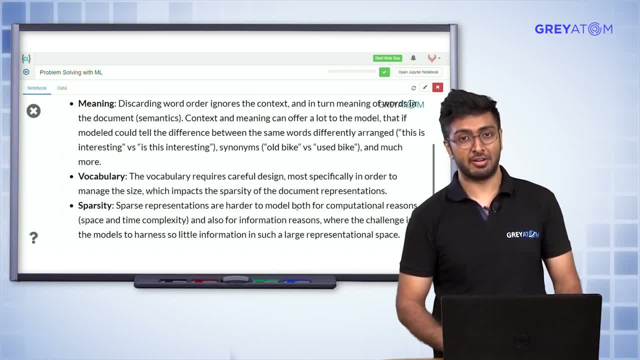 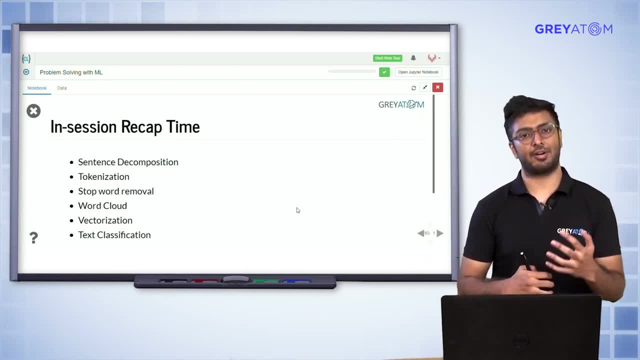 measure and that's something that's a big drawback of bag of words, kind of representations. finally, we are done with the session, so as of now, I have already talked about sentence decomposition. we have talked about tokenization, which is basically sentence decomposition. we talked about how we can use full stop and then we saw 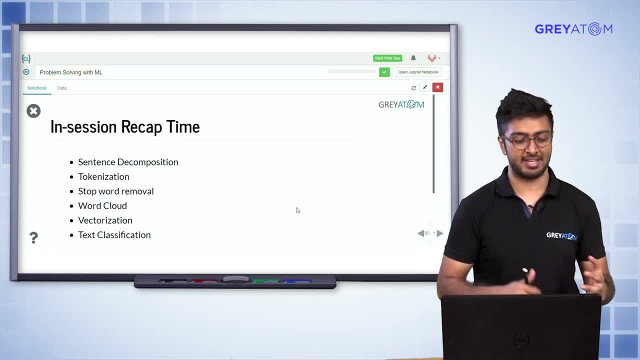 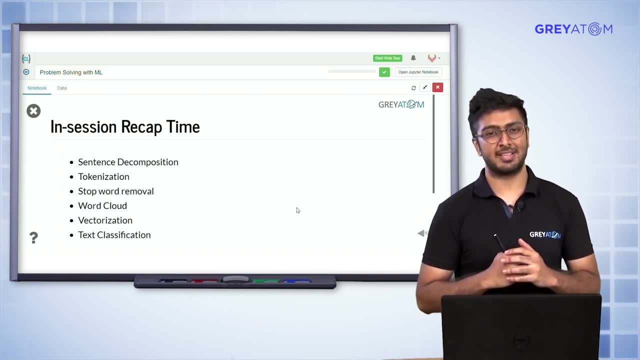 that why full stop was not that using dots it was basically not the best idea and we saw what the solution for that same. with tokenization we could use space to split into different tokens, but then we realized that probably that's not the best way. so we knew about NLDK and its corresponding tokenization. we 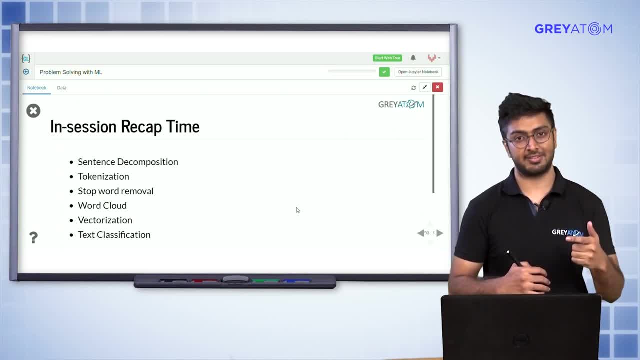 talked about stop-vote removal, we talked about Bort, cloud building, vectorization and finally text classification. so now you are kind of very well covered with what all there is is there in NLP and specifically to text classification. but the one major thing: take away from all. 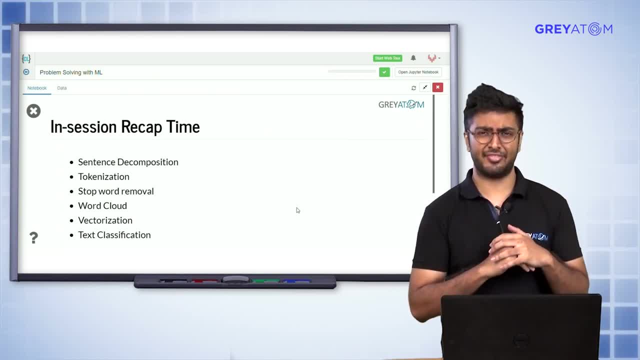 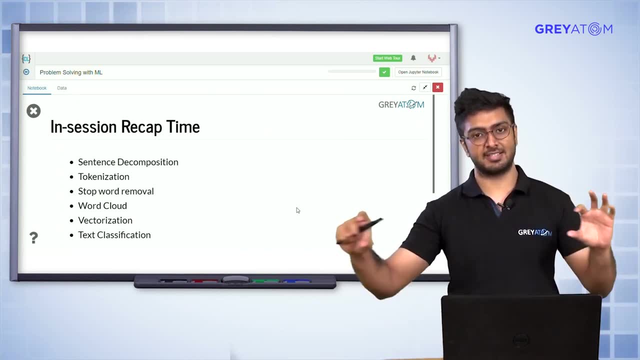 of this lecture is basically the concept of vectorization. that's fairly universal across every LLP task that you would ever do, which is basically taking a text and representing that as a sort of row of vectors, so row of numbers, right? so doing that whole process of vectorization is a pretty nuclear thing. 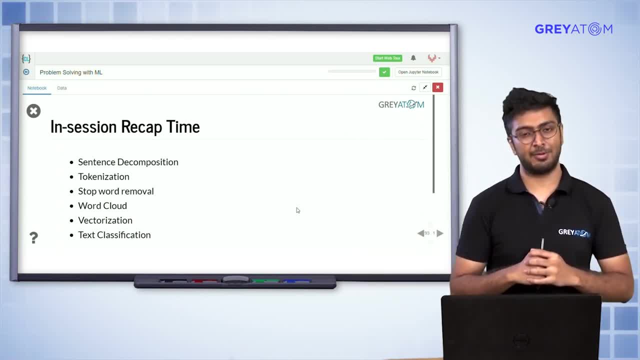 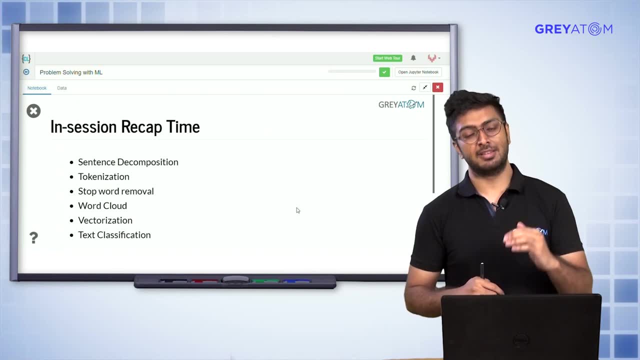 all processes which basically take a text and represent that process of such a sort of row of vectors, so row of numbers, right? so doing that whole process, taking a text to a numeric representation, is crucial for everything that you do, and the best way to do that the you know the amount of effort you. 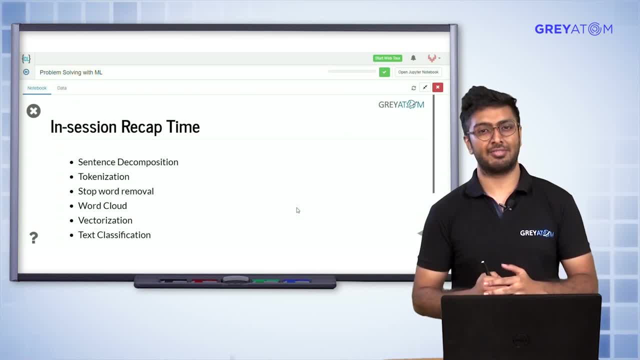 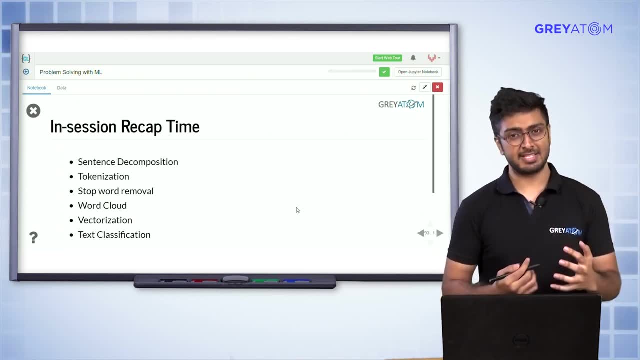 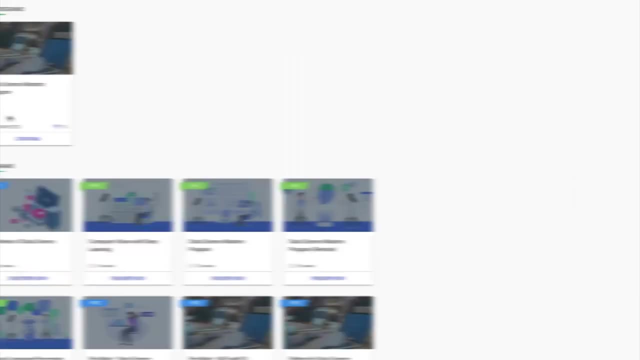 spend doing that. the best possible way is gonna define how well your rest of your text classification or unsupervised learning, is work. it's gonna work, so that's about it. that's a wrap from my again. now let's kind of go ahead and look at the assignments. log on to grey atoms learning platform to unlock more. 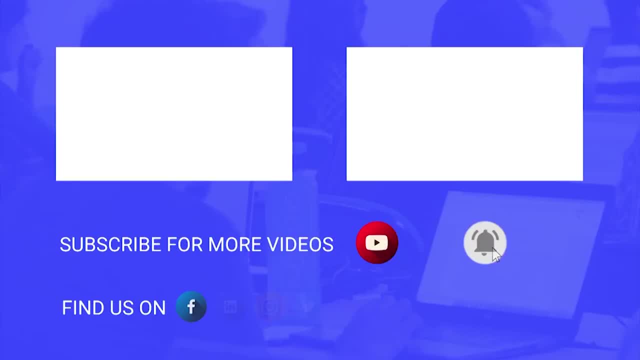 free content. subscribe to our Channel and hit the bell icon for regular updates.